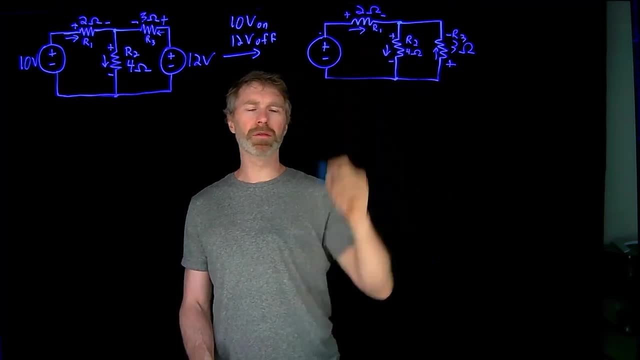 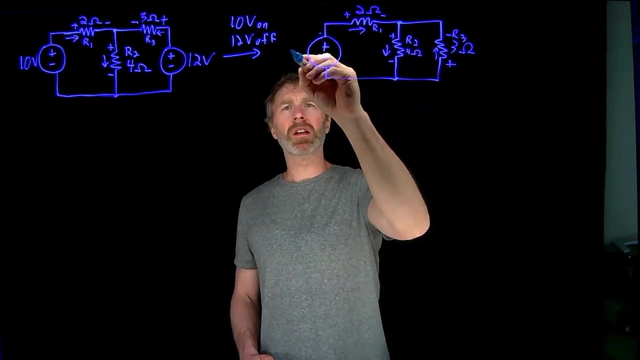 means that this side is more positive than this side and it's plus one volt if I measure in that orientation. So the analysis of this circuit with just the 10-volt source is now fairly straightforward. So the analysis of this circuit with just the 10-volt source is now fairly straightforward. So the analysis of this circuit with just the 10-volt source is now fairly straightforward. 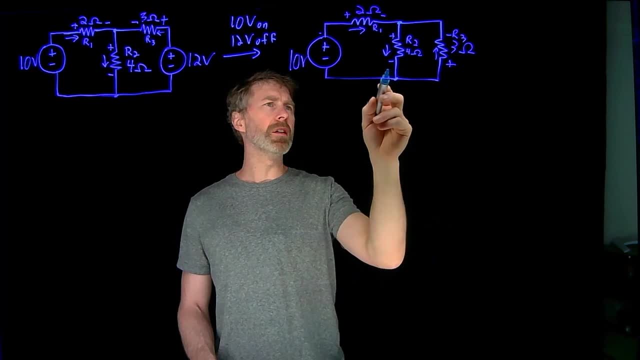 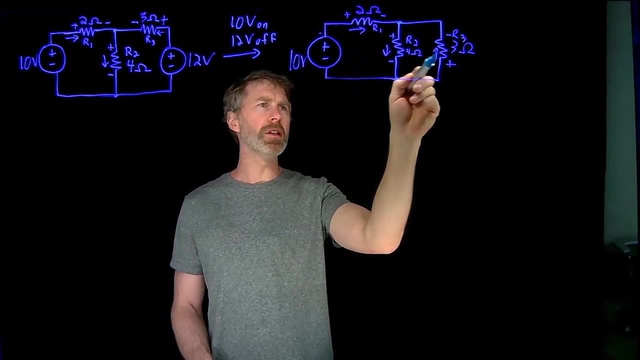 The first step that I can do is combine the R2 and R3. And just to keep in mind, remember, what I'm trying to do is find the voltage across each one of these resistances and then the currents through each one of those resistors. 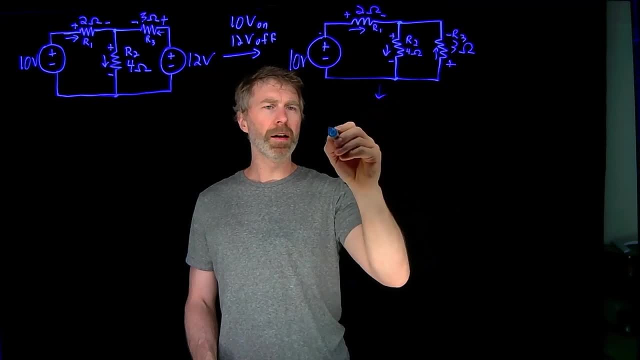 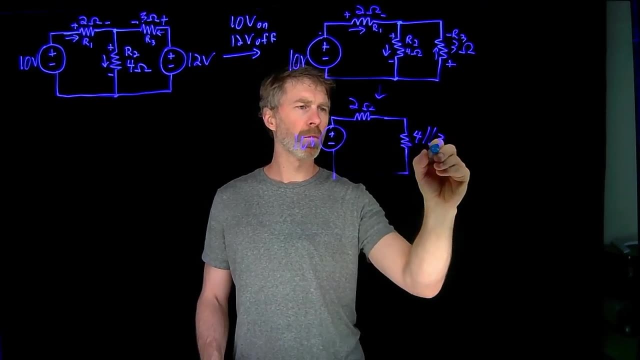 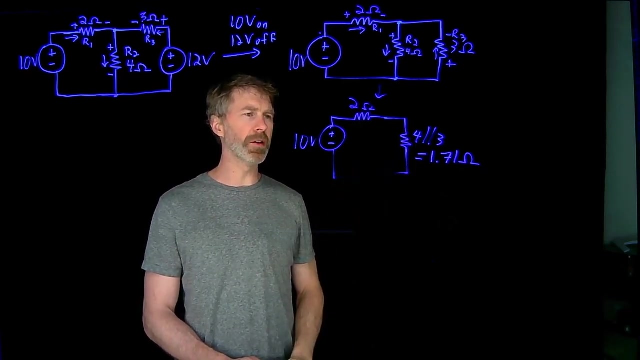 So I can convert that into an equivalent circuit that looks like this: So I've got the equivalent resistance of the 4 ohm in parallel with the 3 ohm resistor. right there, 1.7 ohms is the equivalent resistance. Now I can figure out the voltage Actually. 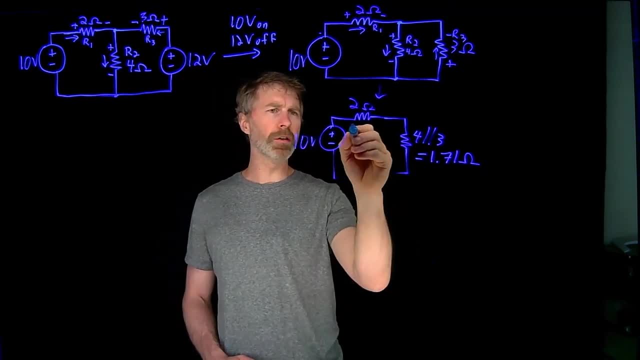 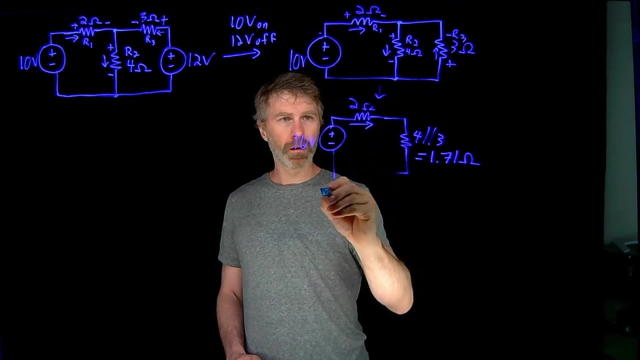 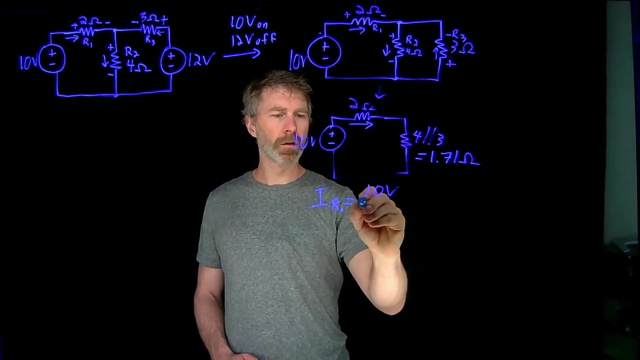 no, let's do the current first. That's the easier one, The current. so the current that's going through R1, and then the equivalent of the 4 parallel with the 3.. We'll call that IR1, because it's the current that's going through R1.. Simply the 10 volts divided by 2 ohms plus 1.71 ohms. 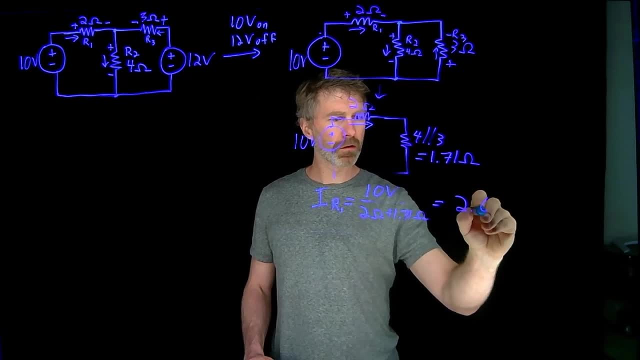 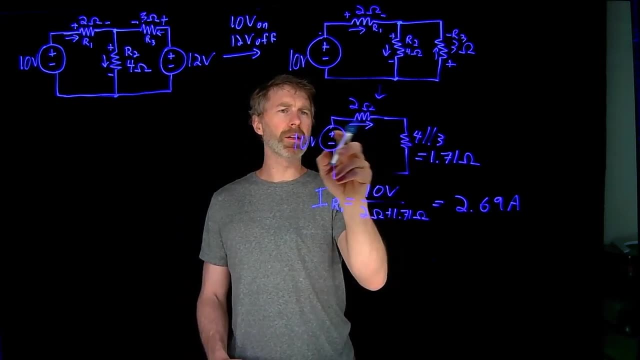 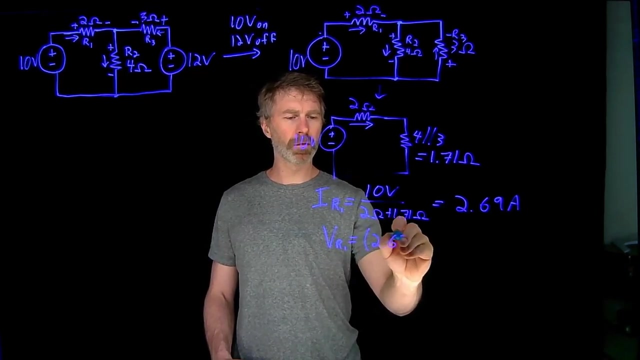 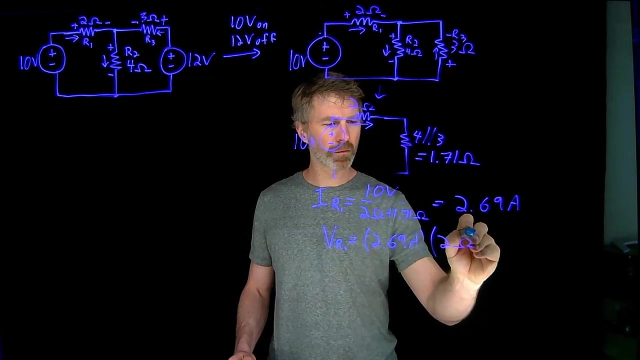 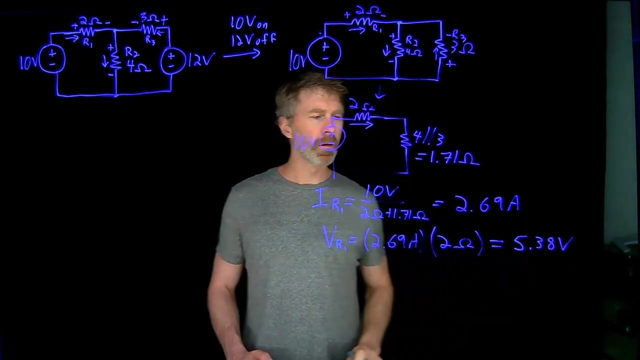 And that works out to 2.69 amps. The next thing I can figure out is the voltage across R1, because I now know the current that's going through it And I can simply take that current 2.69 amps and multiply by the resistance. Okay, so I've got 5.38 volts across that 2 ohm resistor. Now, if I 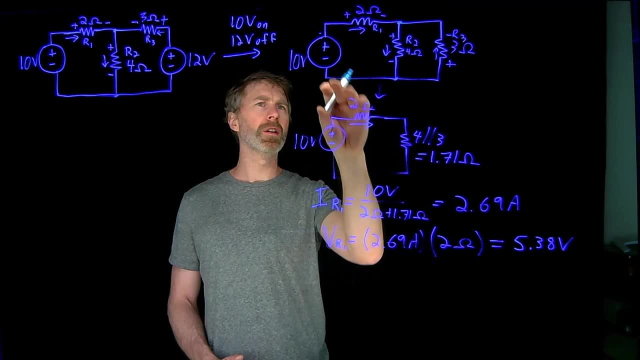 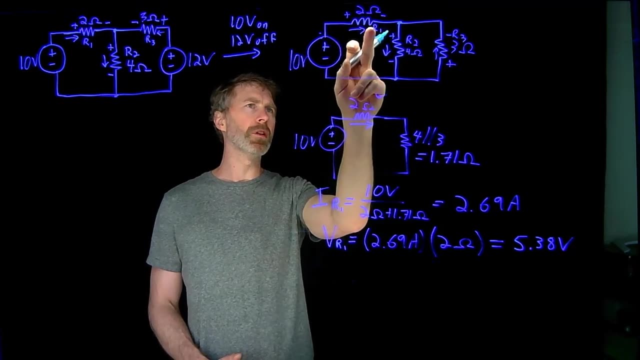 go back to this original circuit with a 10 volt on the 12 volt off, I've got a 10 volt source and now I have 5.38 volts, a drop across the 2 ohm resistor. Whatever is left over is the voltage. 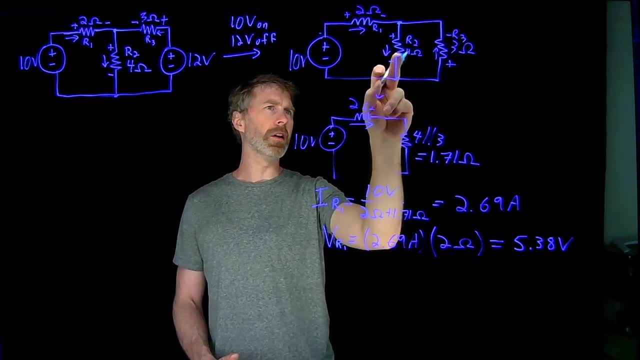 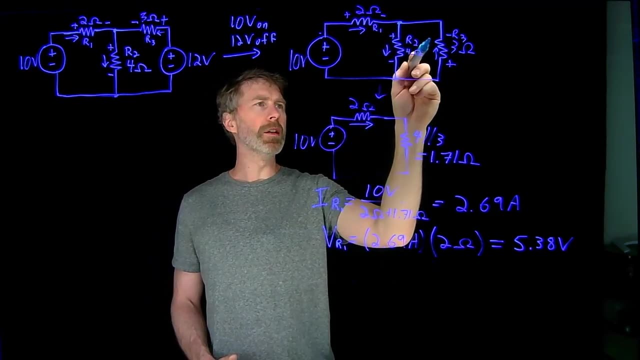 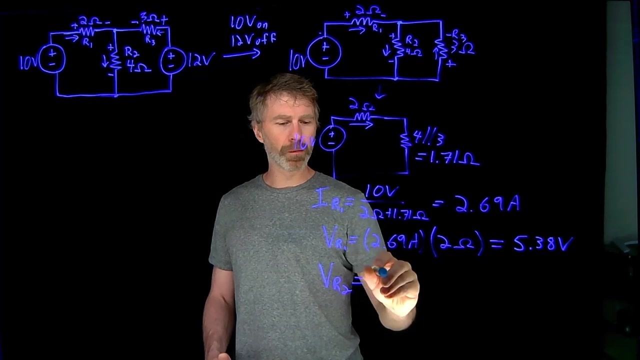 across R2 and across R3.. The way I've defined voltage here is: the voltage for R2 is positive here, negative here, and the voltage for R3 is negative here and positive here. So let's go V- R2 just using Kirchhoff's voltage law, It's the 10 volts from the source. 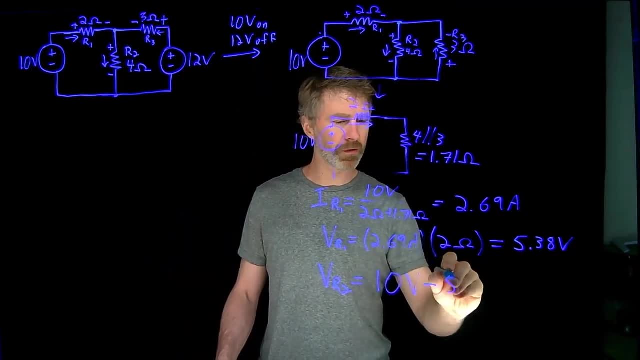 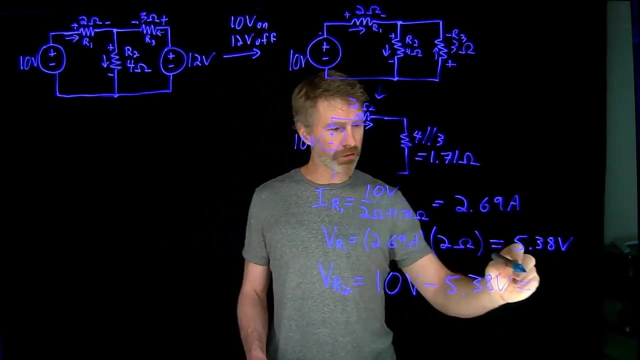 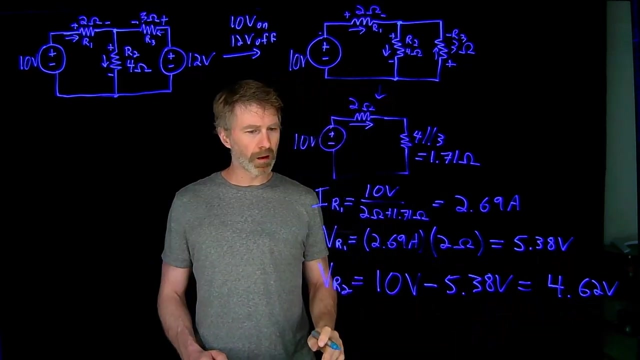 minus the drop across that 2 ohm resistor, which we've just calculated to be 5.38 volts, and that works out to 4.62 volts, and V R3 is just the R2 and R3 are in parallel with each other, so 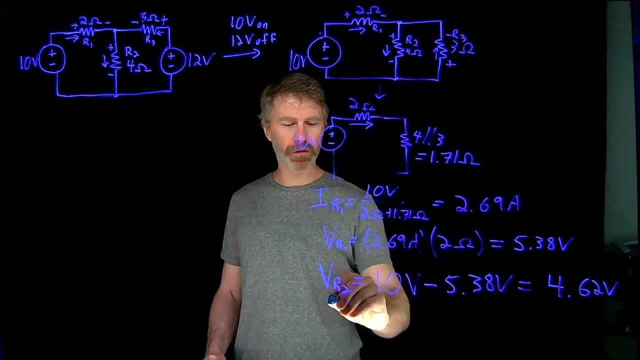 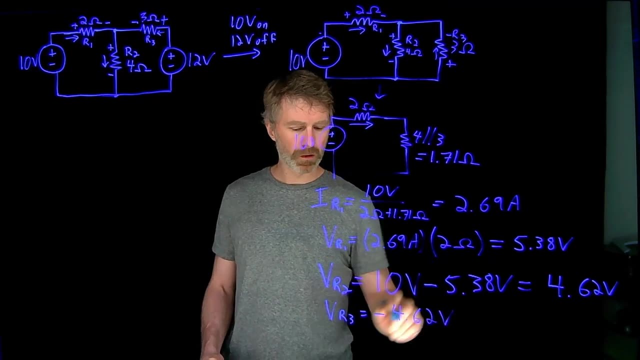 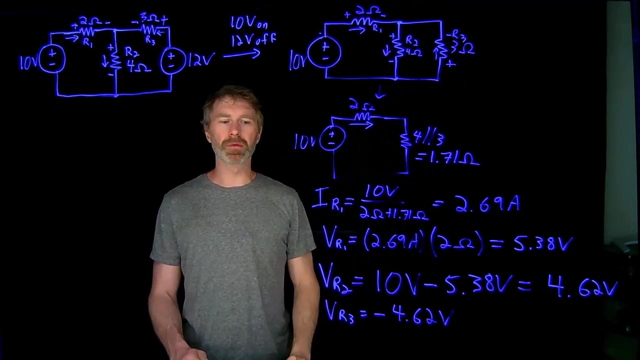 V R and V R3 is just going to be the negative of V R2.. Okay, and now that I've got the voltages across those two resistors, pretty easy- easy to figure out what the current through those resistors are. It's just going to be the voltage divided. 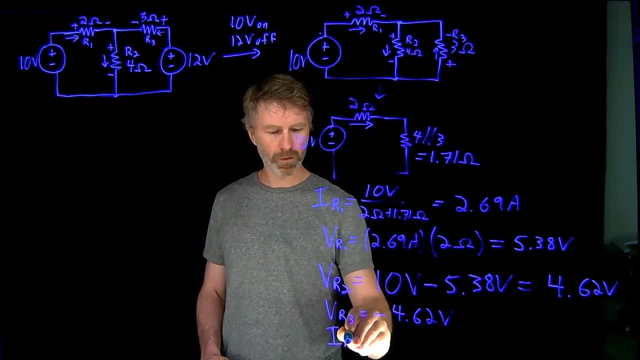 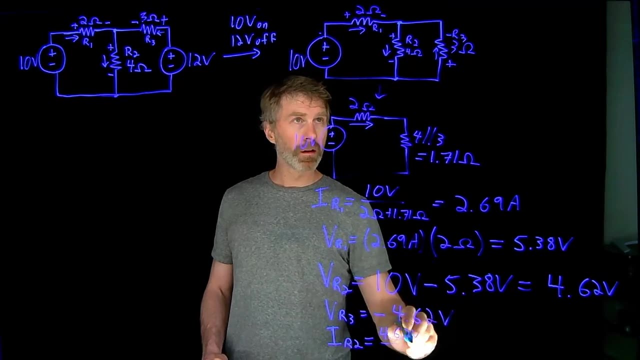 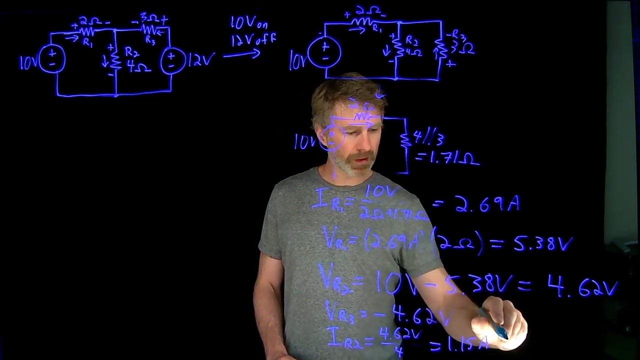 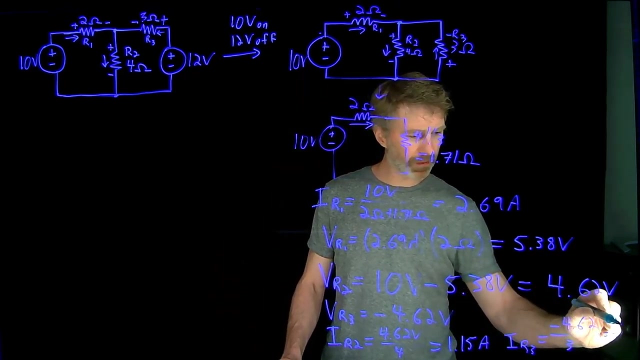 by the resistance. So IR2 will be that 4.62 volts divided by 4 ohms, 1.15 amps, And IR3 and that works out to negative 1.5 oh. I'm kind of running out of space there. I'm going to write it. 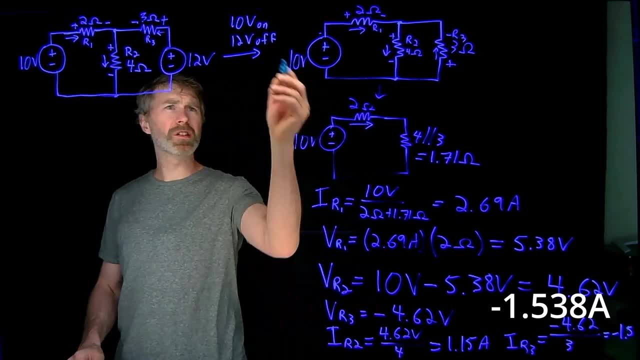 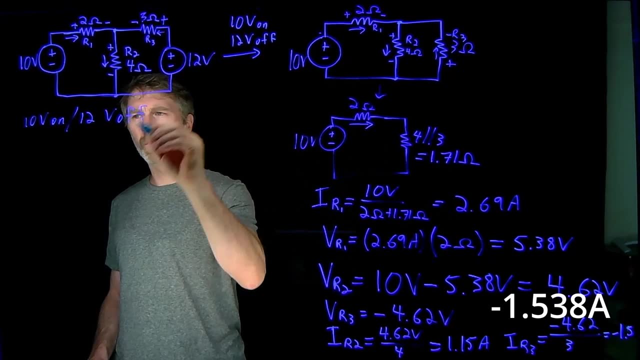 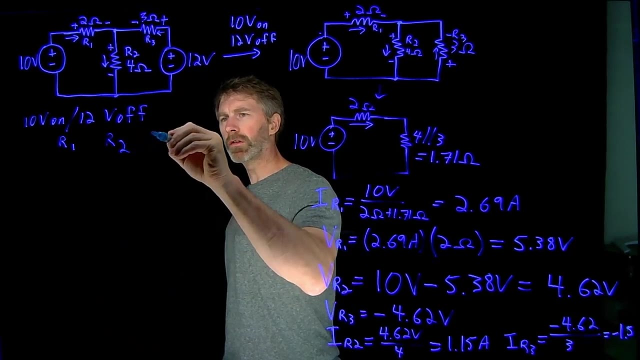 over here because I got to. I'm going to create up a table anyway. So for this case, one of 10 volt on 12 volt off, we have our three resistors, R1, R2 and R3, and we've just calculated the voltage and current for them. 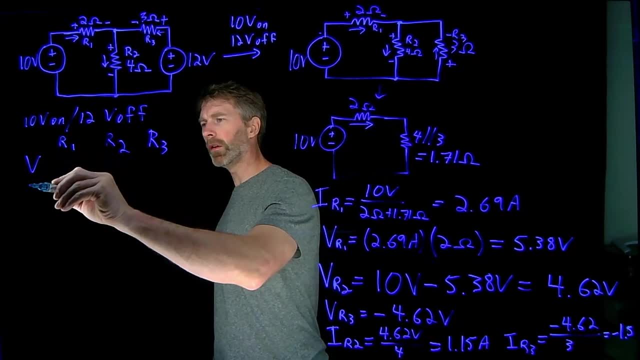 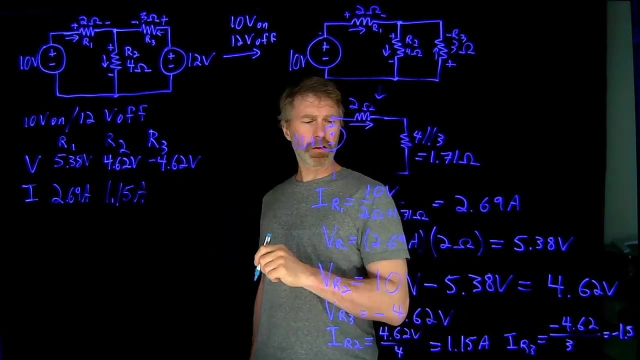 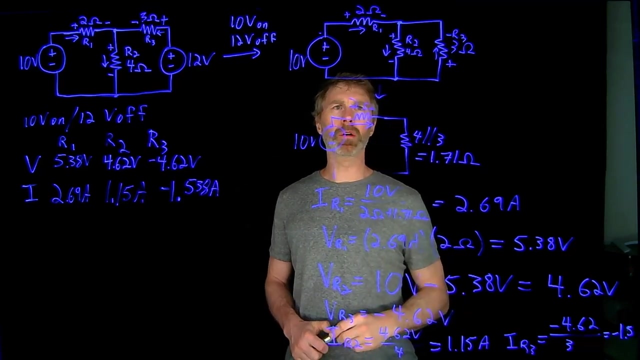 Okay, so that's the full analysis, getting all the voltages and currents for R1, R2 and R3.. In the case when the 10-volt source is ON and the 12-volt source is OFF. Now let's look at the second half of the superposition. 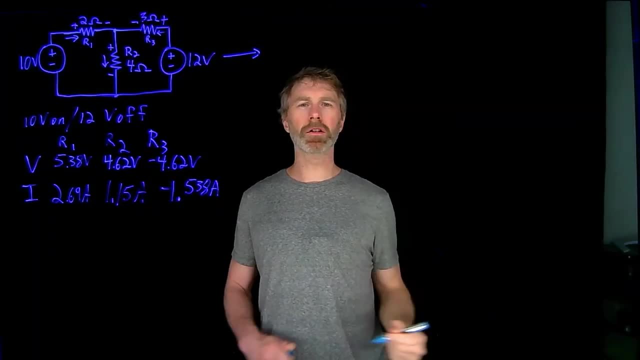 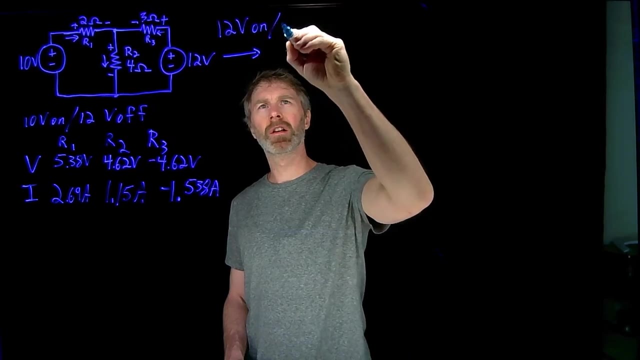 Now let's look at the second half of the superposition. Now let's look at the second half of the superposition. Now let's look at the superposition where the 12-volt source is on and the 10-volt is off. 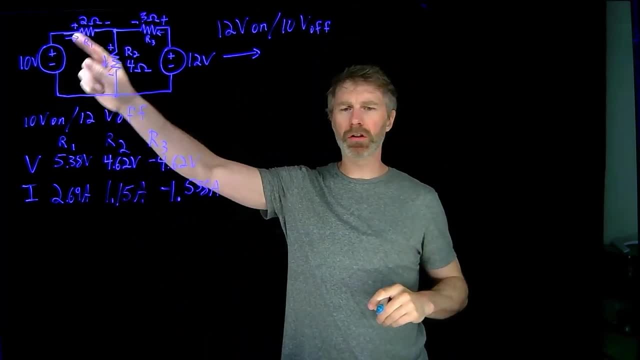 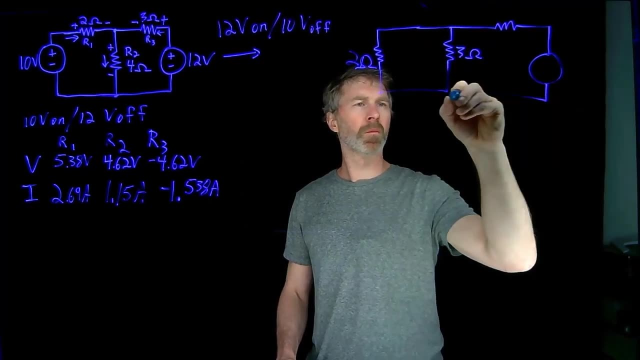 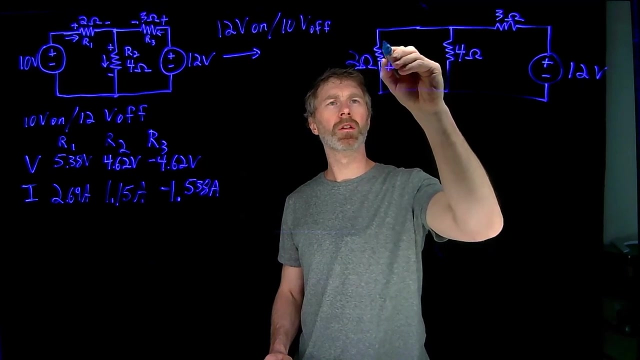 So that means the 10-volt gets dialed down to zero. That just becomes a short circuit and I can redraw the circuit here. Now let's redraw the polarities and current directions for each one of these resistors. So I've defined the current as that orientation and the voltage in that orientation. 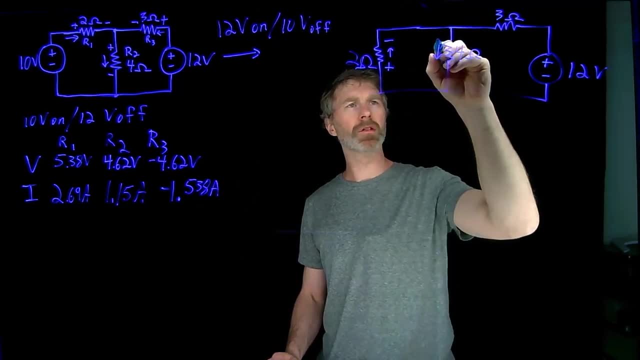 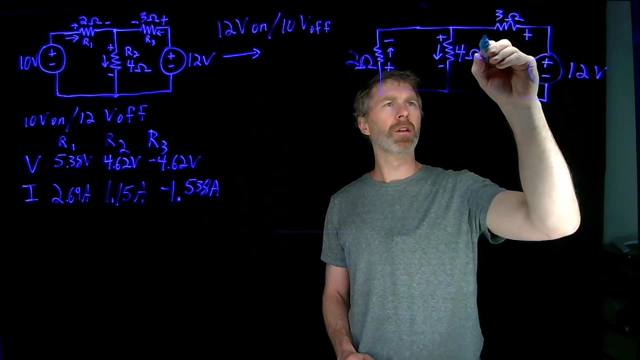 the current going up here, the 4-ohm resistor. the current's going that direction and I've got the voltage defined in that orientation. For the 3-ohm resistor, voltage is like that and the current is going in that direction. 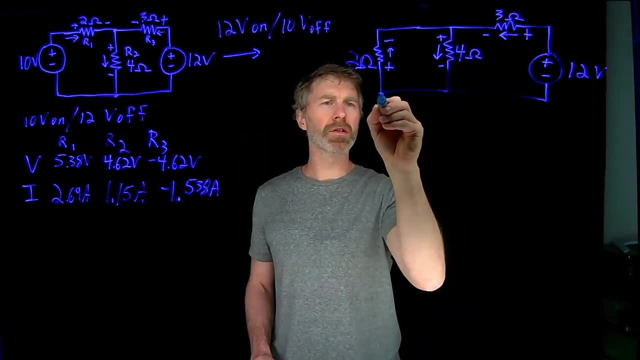 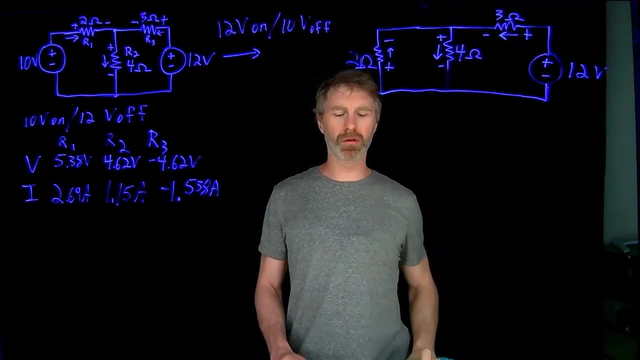 So this is actually the steps for the analysis of this circuit. It's pretty much identical to what it was for the 10-volt circuit. I just have a 12-volt. I have the 10-volt source over on this side instead of the 10-volt source over on this side. 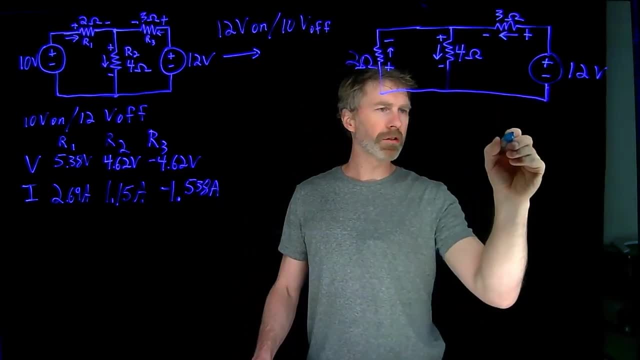 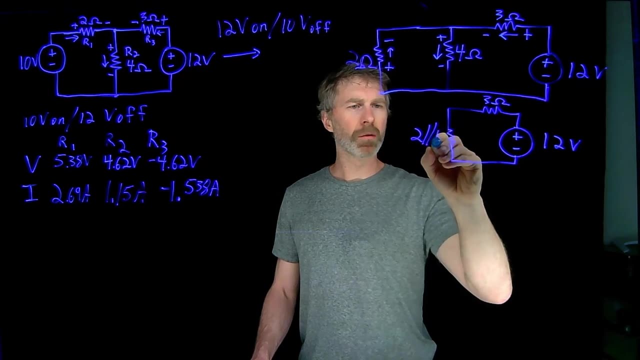 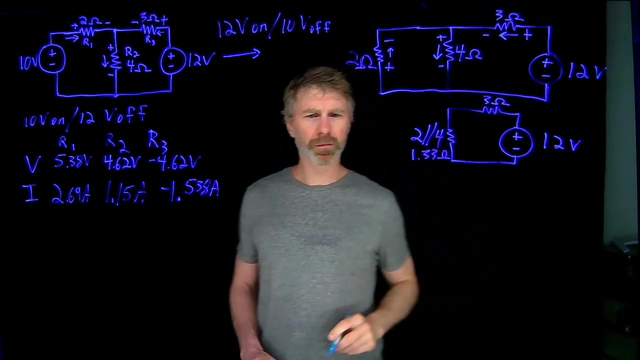 So again, it's a fairly simple process. I can redraw the circuit to make it easier to analyze. This is a 2-ohm in parallel to a 4-ohm resistor, which is 1.33 ohms. Now I can figure out the current through R3 here. 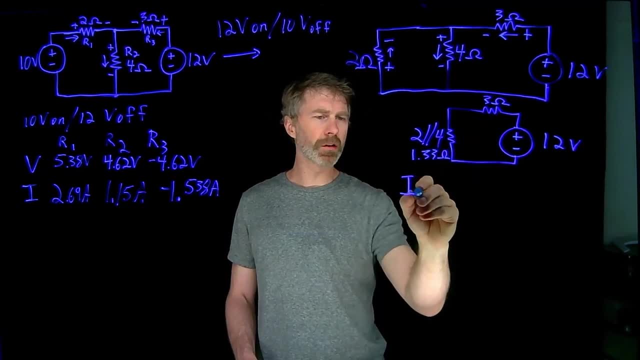 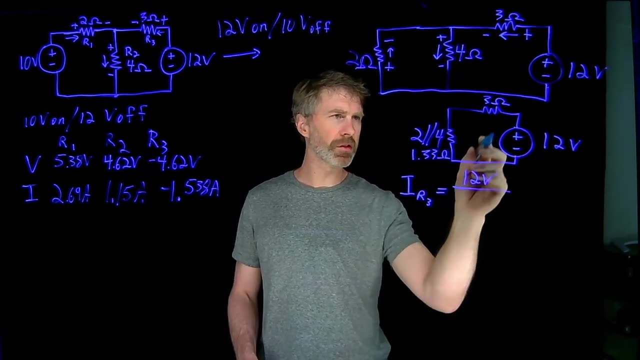 It's going to be the current. It's going through R3.. It's going through R3. It's going through R3 in this equivalent circuit. So it's 12 volts divided by the total resistance of this series circuit. 3 ohms plus 1.33 ohms gives me 4.33 ohms. 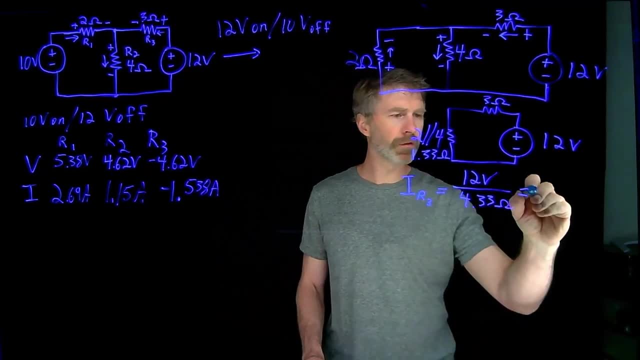 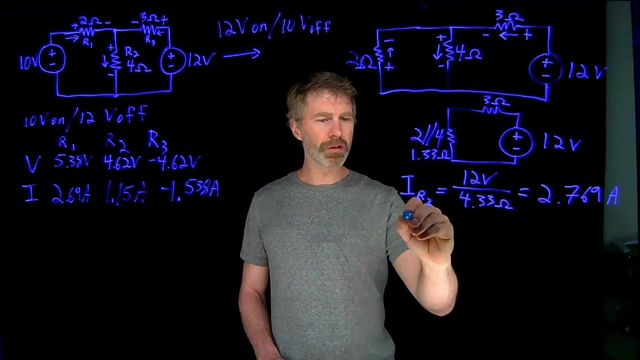 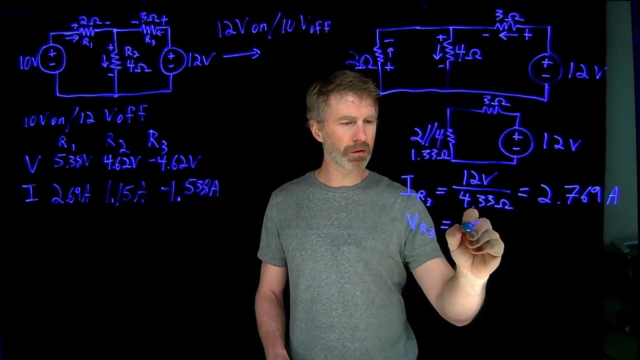 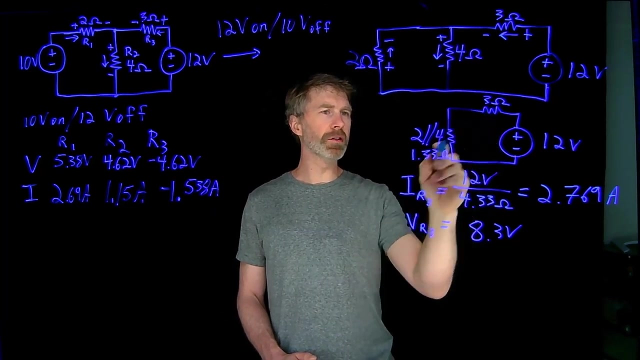 and a current of 2.769 amps, And then the voltage across R3 is simply going to be that current 2.769 times the 3 ohms, And that works out to 8.3 volts. Now again, if I have 8.3 volts across this 3-ohm resistor, 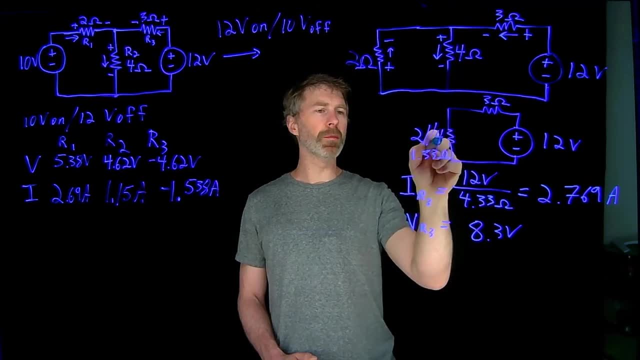 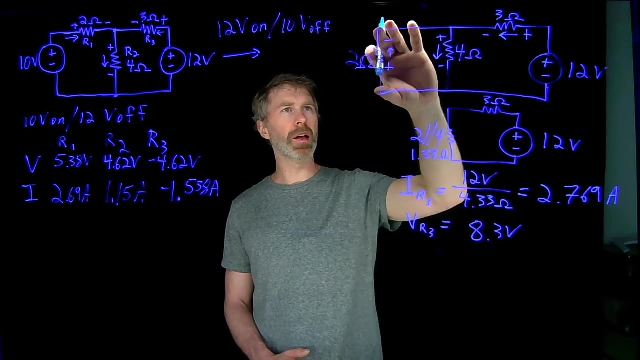 whatever's left over will be what's across this parallel combination, Or the other way to look at it, is going back to this original circuit. here It'll be the voltage across the 4-ohm resistor and the voltage across the 2-ohm resistor. 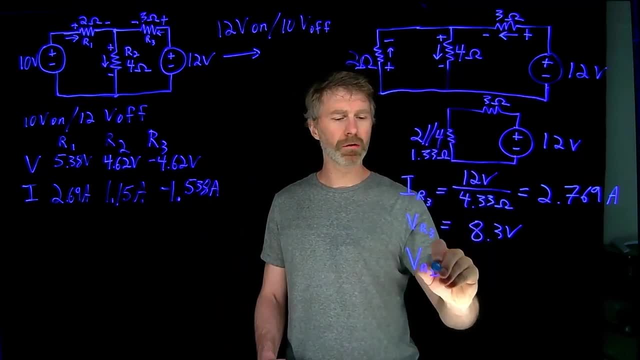 So this one is R2.. So VR2, because the orientation of the polarity that I've defined there is the same as what's across the 3-ohm resistor. So VR2 is simply going to be the 12 volts minus what I've just calculated for that R3.. 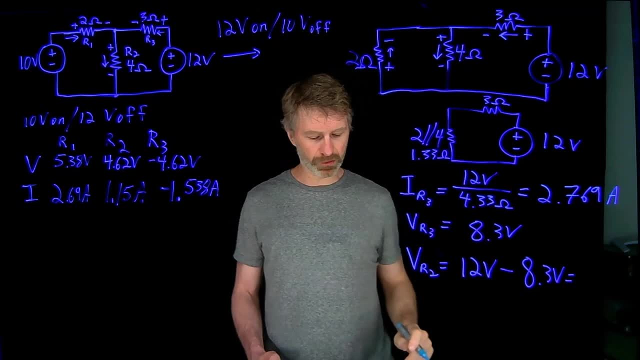 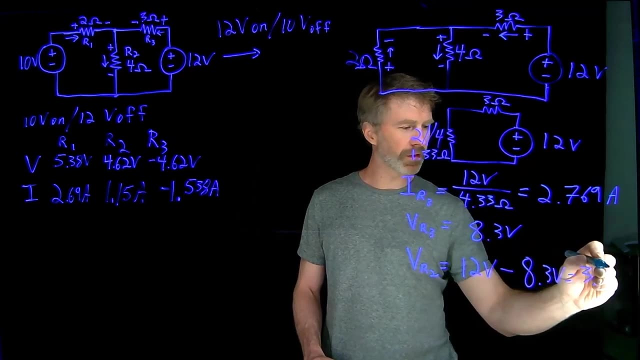 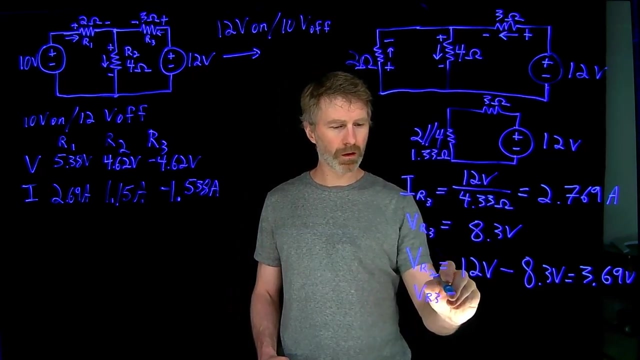 8.3 volts And that works out to Well. I did some rounding in this, so it's actually going to be 3.69 volts. Without that rounding, VR3 is the Opposite or the inverse of that, so it's negative 3.69 volts. 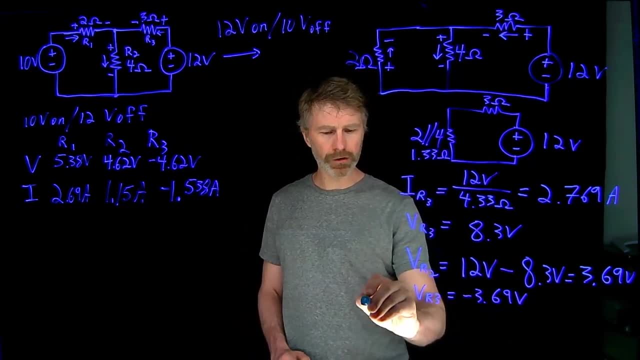 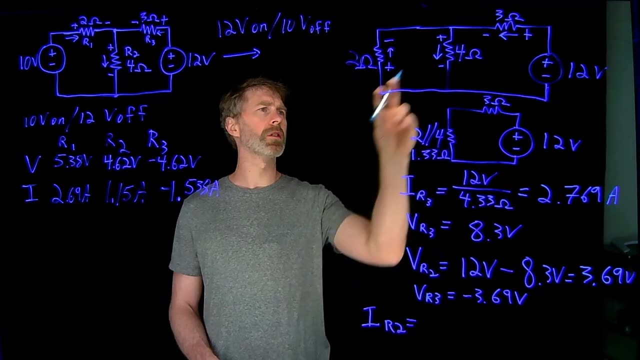 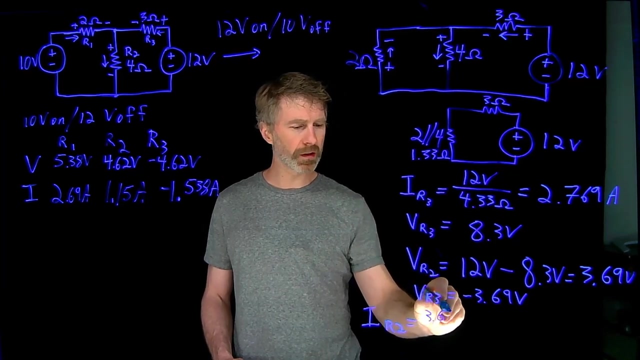 Now I need to figure out IR2 and IR3.. Well, IR2.. We know the voltage across the 4-ohm resistor and we know the resistance of it, so it's simply going to be that 3.69 volts divided by 4 ohms. 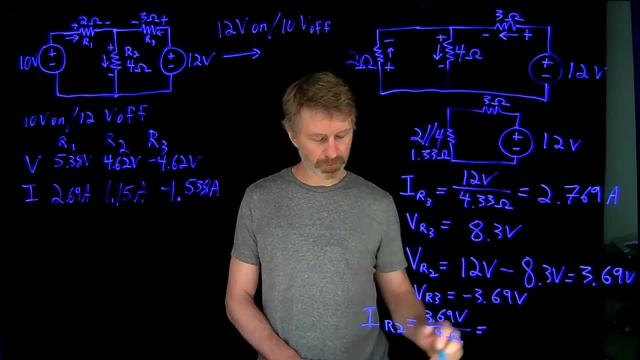 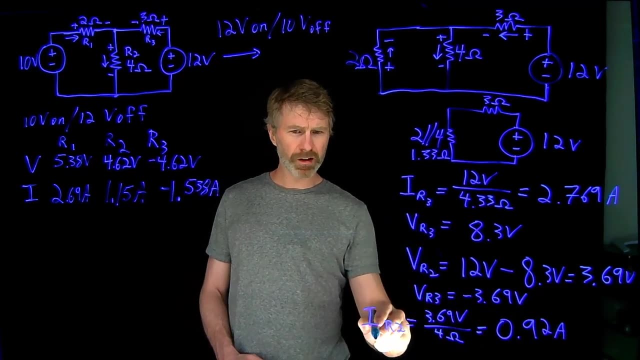 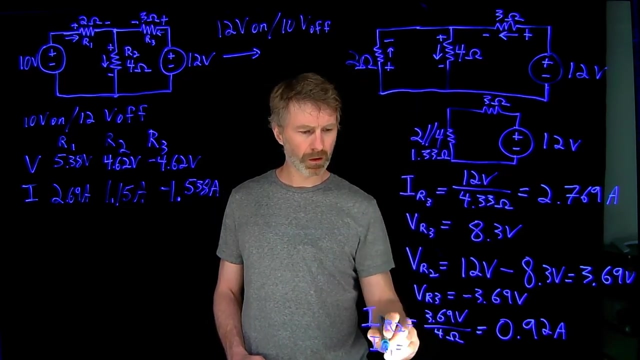 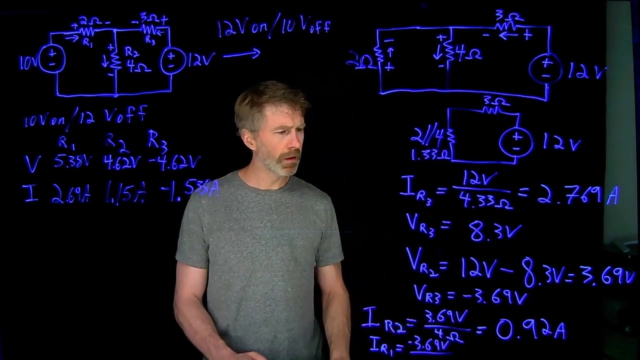 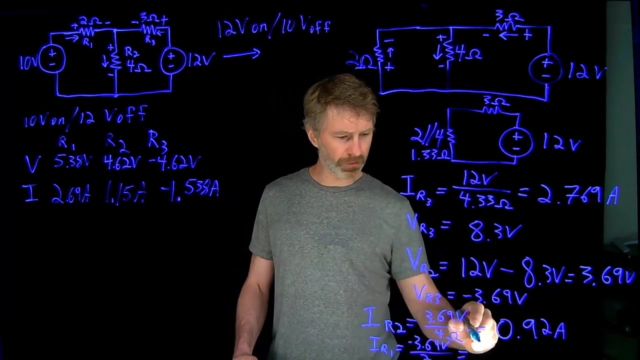 And that works out to 0.92 amps. And then IR3.. No, IR1. is also 3.69 volts, but the other polarity divided by the resistance of it, that's 2 ohms, And that works out to negative 1.845 amps. 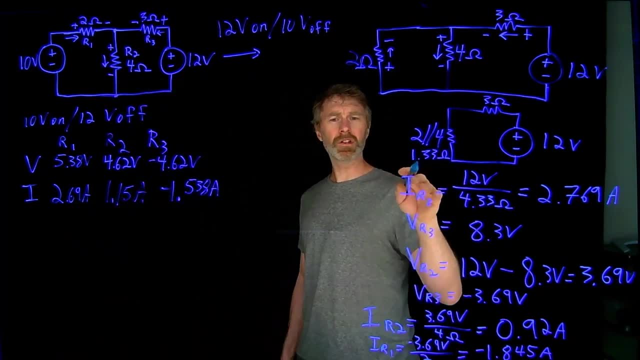 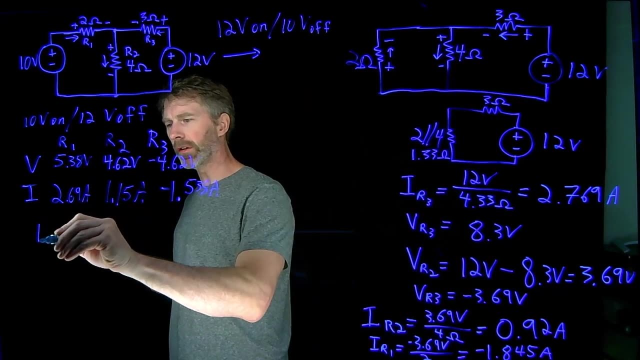 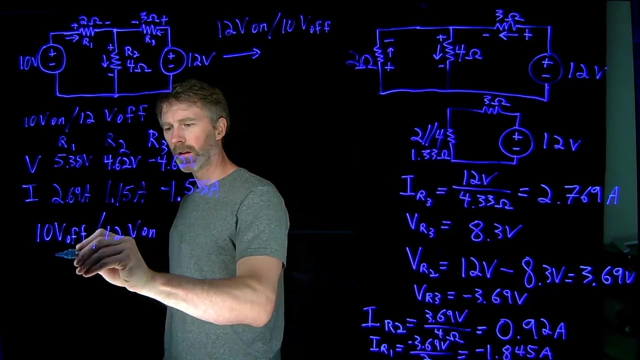 So now I've figured out the voltage and current for each one of these resistors in the second case here. So this is the case where the 10 volts off and the 12 volt source is on. So I've got R1,, R2, and R3. 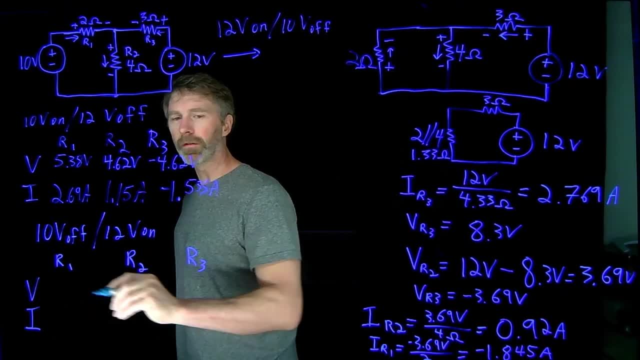 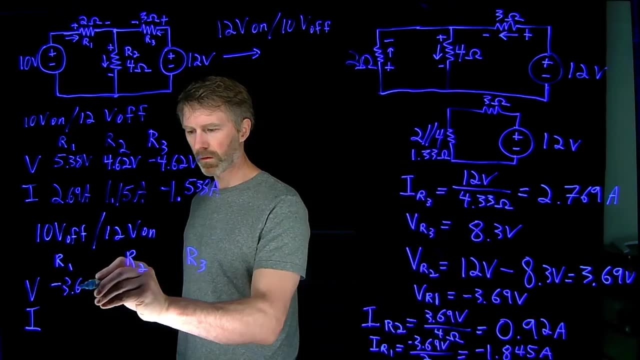 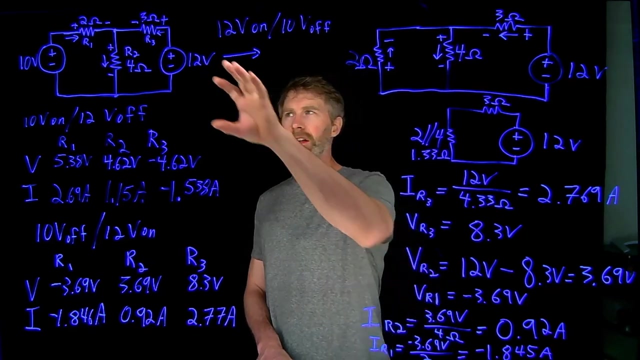 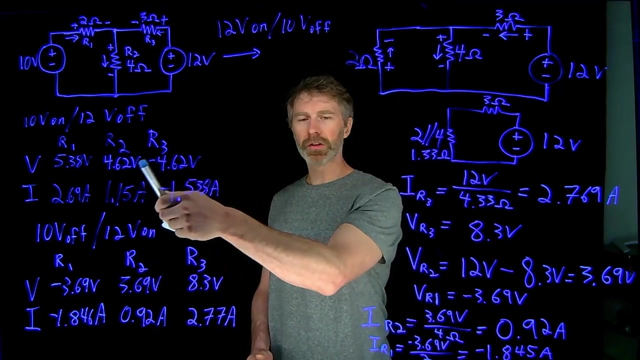 And I've got the voltage and the current values for each one of those. Now I'll just fill in the table here And now. in the initial circuit, the voltages and currents for each one of those resistors will be the sum of the voltage and current from this table. 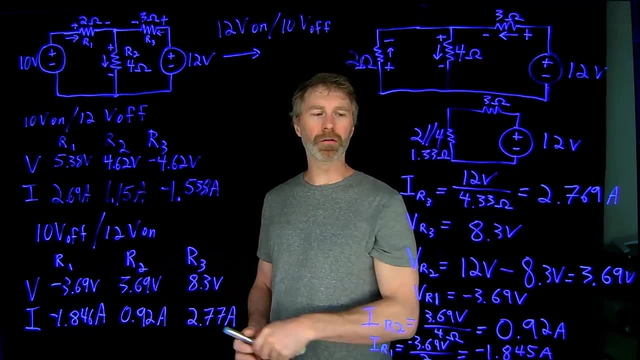 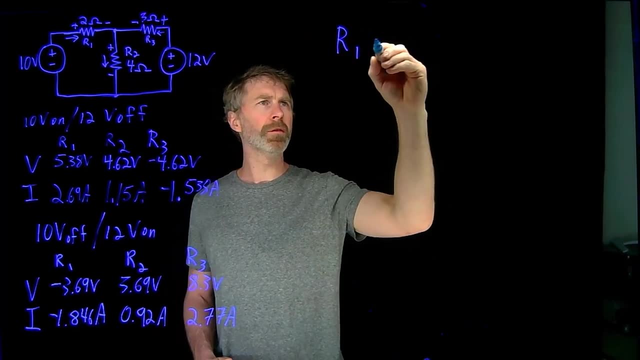 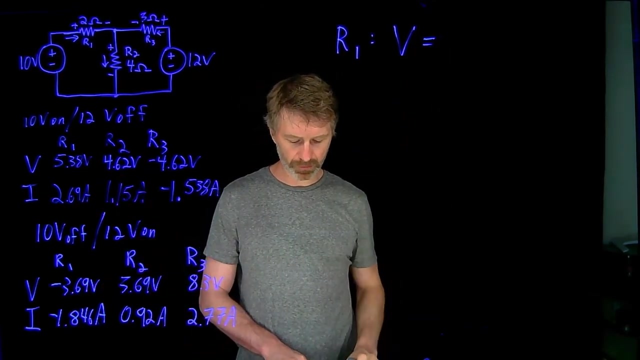 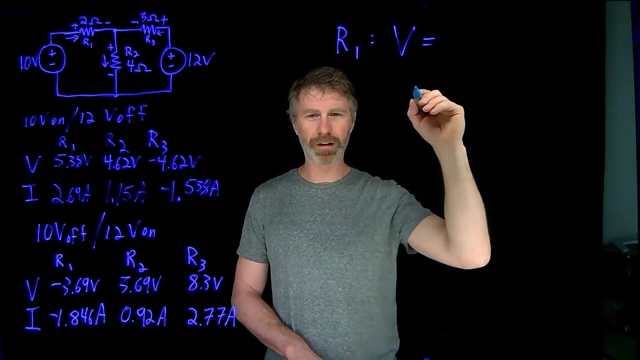 and the voltage and current for this table. So overall for R1, the voltage will be 5.38 plus negative 3.69.. I just don't totally trust what I've got here. I've got 1.69 volts. 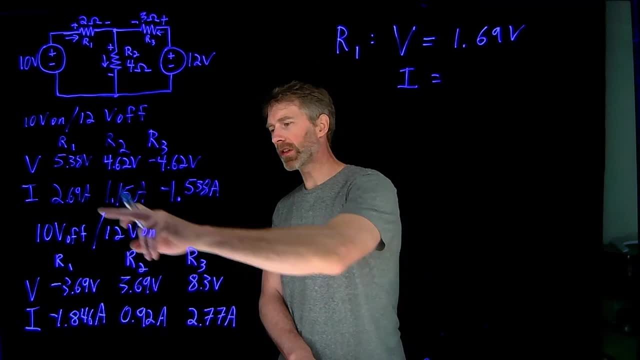 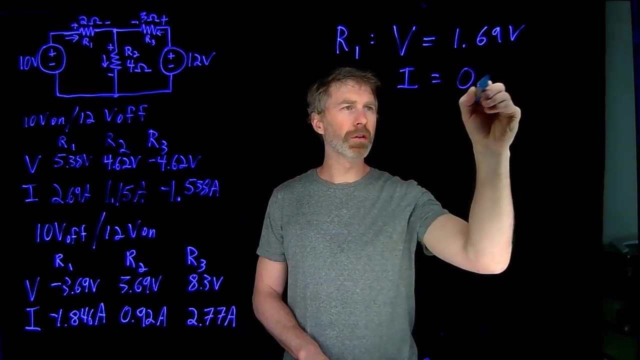 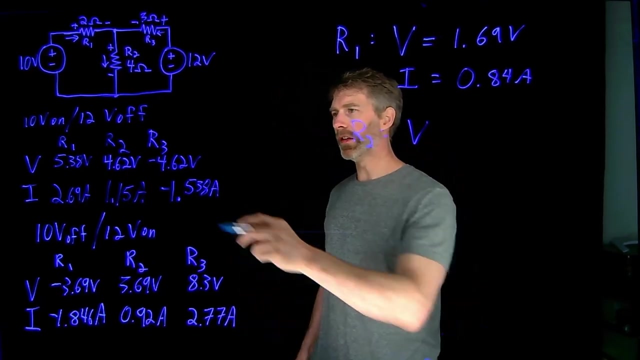 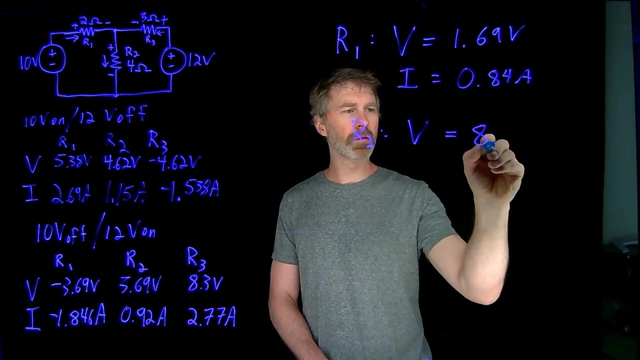 And the current through it is 2.69 amps Plus negative 1.846 amps, which gives me 0.84 amps, And then for R2, the voltage is 4.62 volts plus 3.69 volts, Gives me 8.31 volts. 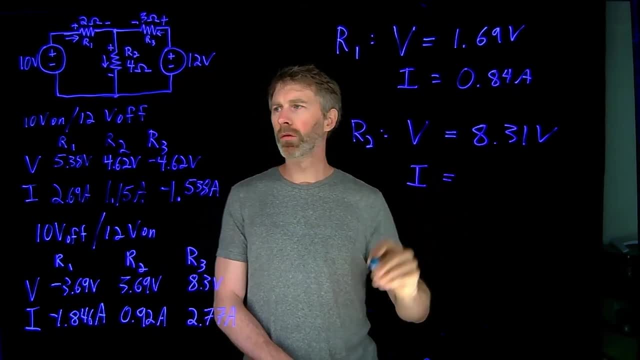 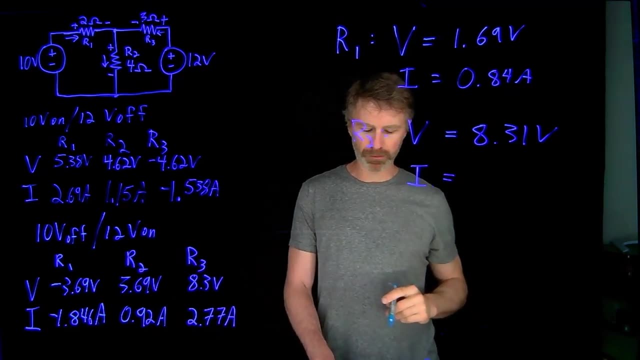 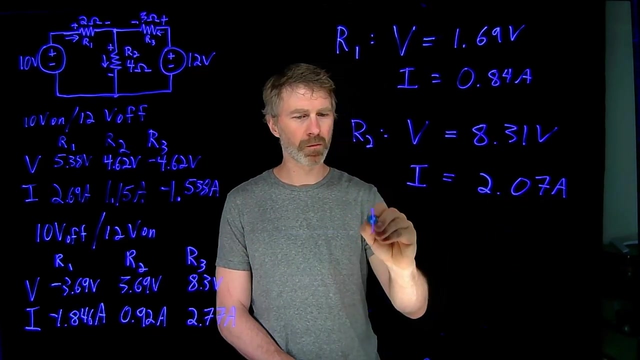 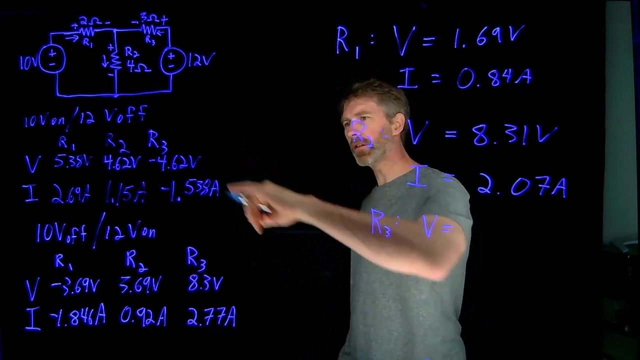 And the current through R2 will be 1.15 amps from the first circuit Plus 0.92 amps from the second circuit, And then for R3, the voltage across R3 will be the negative 4.62 volts plus 8.3 volts. 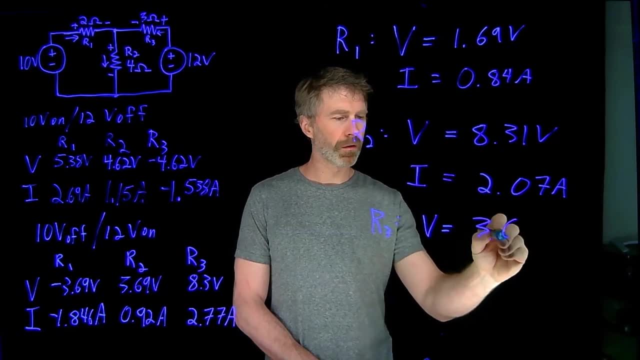 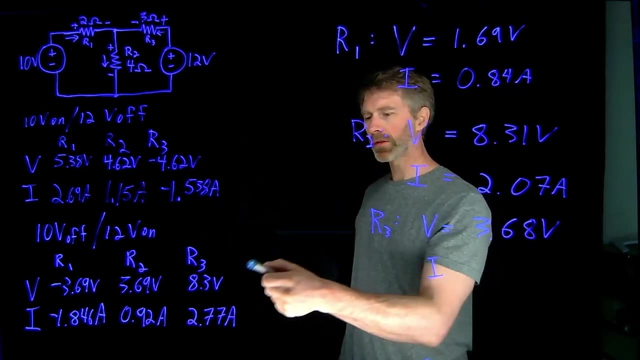 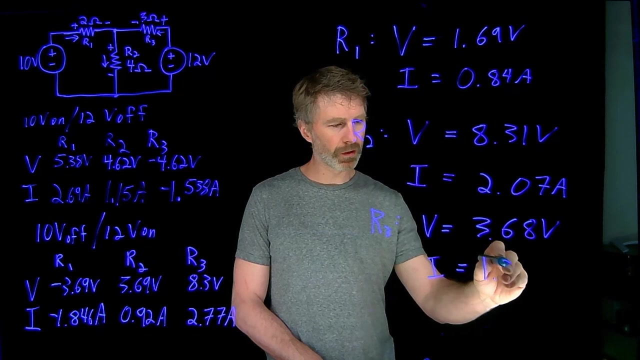 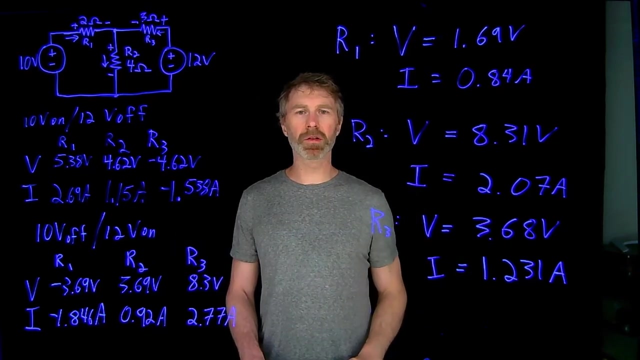 And that works out to 3.68 volts And the current through it is negative 1.5 volts. So that's negative 1.538 amps plus 2.77 amps, Which works out to 1.231 amps. Okay, that was an example of the superposition principle. 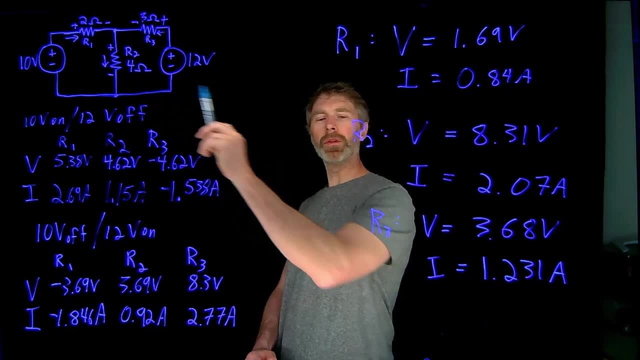 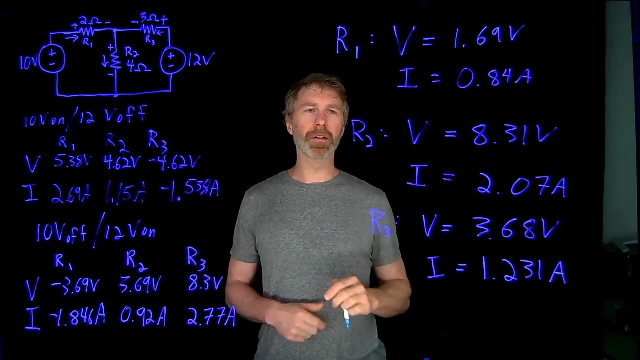 in action for a simple circuit with only two voltage sources. So we have two different circuits to analyze and then take the results from those two circuits, combine them together and that gives us what's in the actual original circuit. So thanks very much for watching. 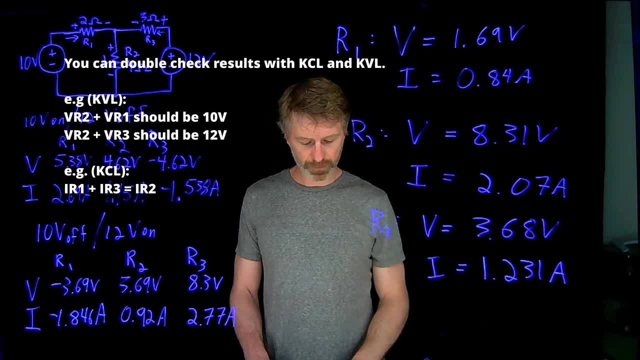 See you in the next video. Okay, I think I copied down right what I got here up to here. Hopefully those calculations were correct, See ya.